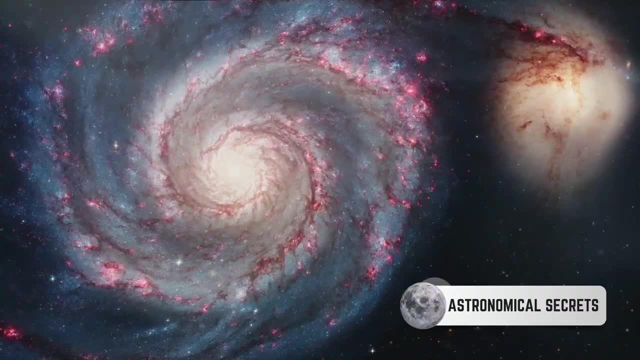 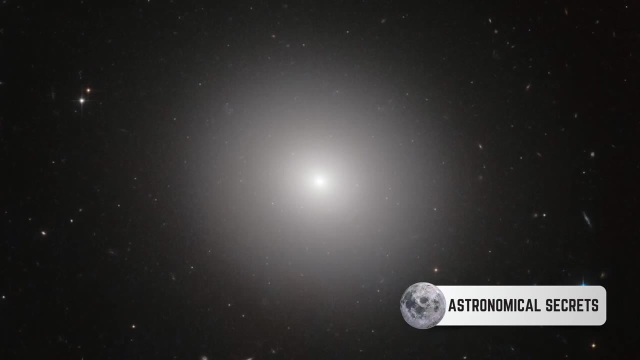 They're like the quiet elderly relatives of the bustling lively spirals, having used up most of their gas to form stars long ago. Their serene appearance, however, belies the immense gravitational force they wield, binding together up to a trillion stars. So are these galaxies just? 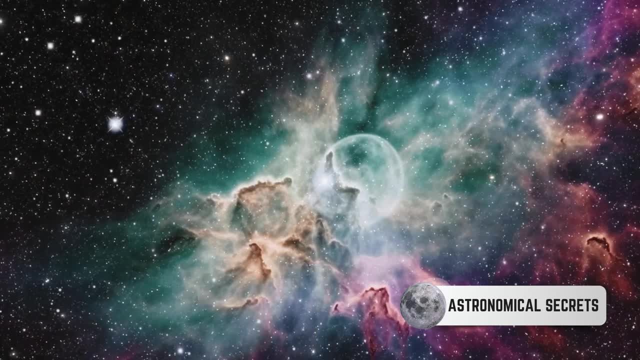 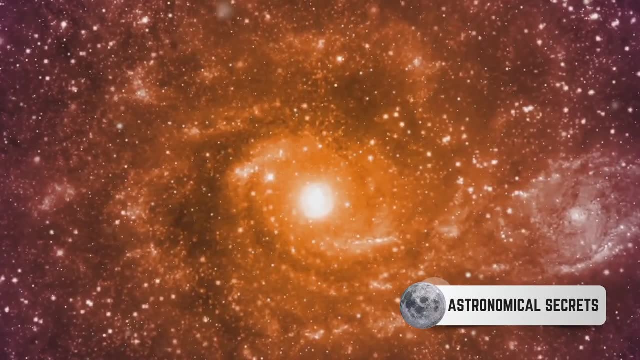 quietly napping, or is there more to these cosmic giants than meets the eye? Stick around to find out. Elliptical galaxies are like the eggs of the universe. They come in all sizes, from small to humongous. These cosmic omelets, if you will, sport a shape that is three-dimensional. 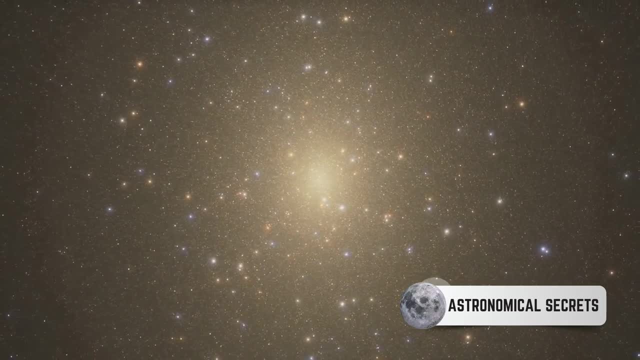 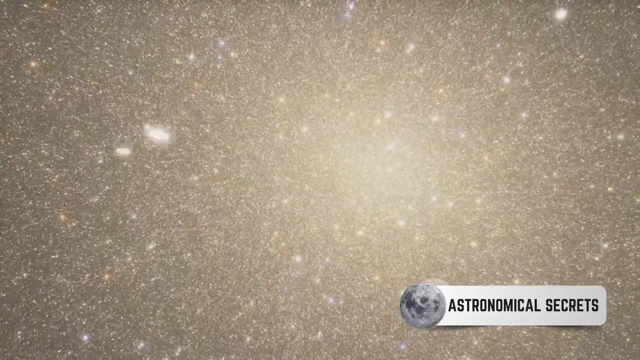 and ellipsoid, similar to a flattened sphere or a squashed ball. Imagine a beach ball that's been sat on and you'll get the idea. Now these galaxies are quite the rule-breakers when it comes to size. Some are petite little things called dwarf ellipticals that are a mere few. 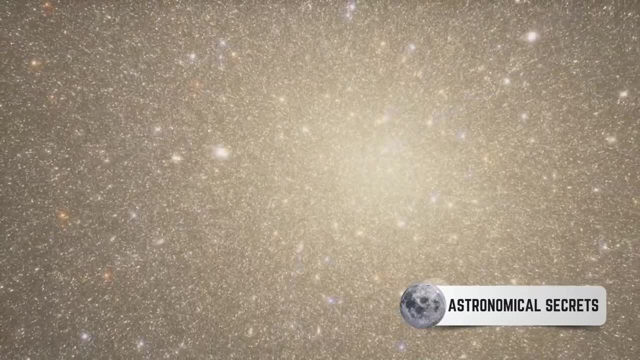 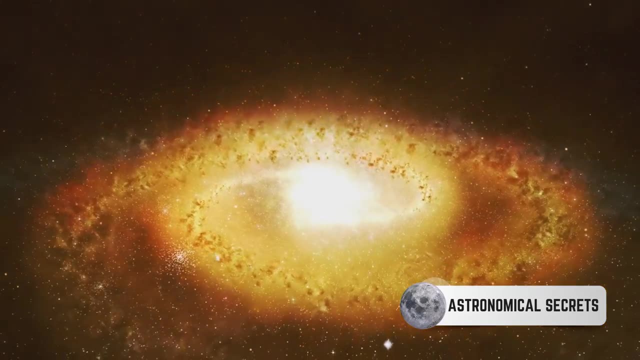 thousand light-years across. On the other end of the spectrum, we have the giant ellipticals. these are the real showstoppers. stretching across several million light-years, That's a lot of space to fill. But what fills that space, you ask? Well, elliptical galaxies. 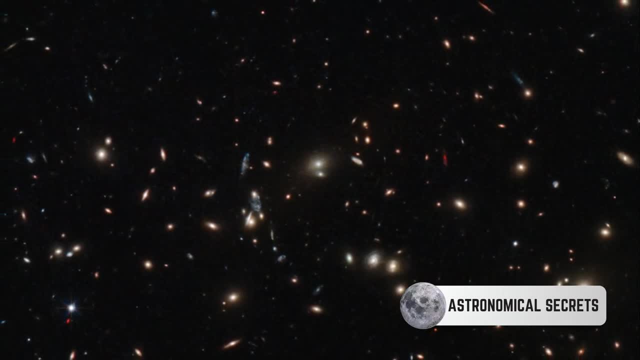 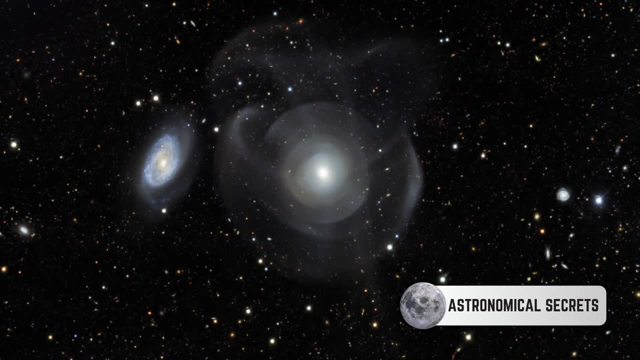 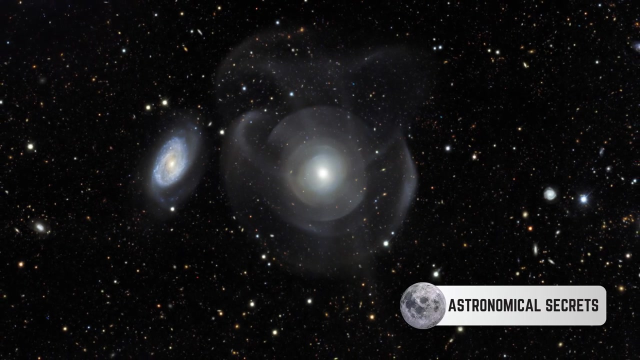 are brimming with older stars. Unlike their spiral siblings, these galaxies don't have the spiral arms that we often associate with galaxies. These arms are the birthplaces of new stars, meaning elliptical galaxies aren't producing many new stars. Instead, they're filled with mature stars that have been around the cosmic. 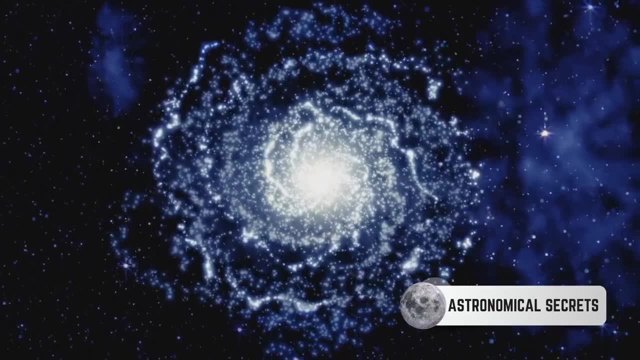 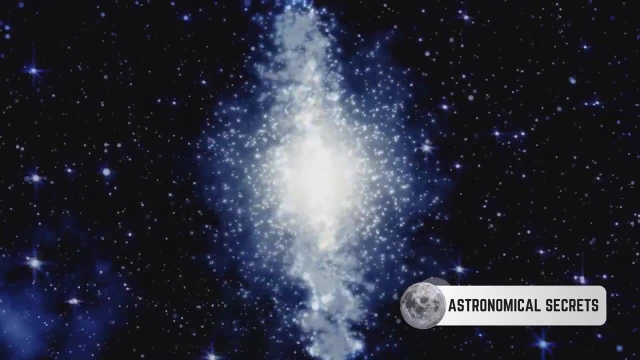 block a few times. And that's not all. Elliptical galaxies are also chock-full of globular clusters. These are tightly-packed groups of stars that orbit the galaxy's center like bees buzzing around a hive. Each of these clusters can contain hundreds of thousands of stars, adding to 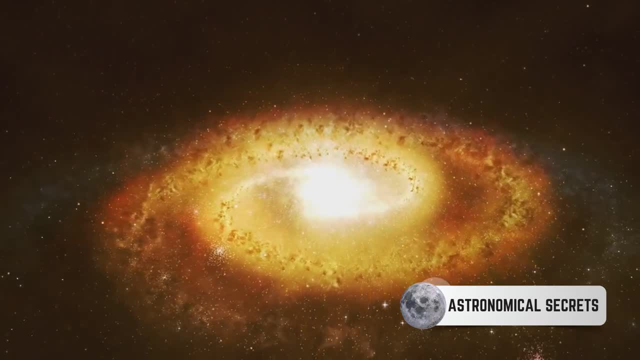 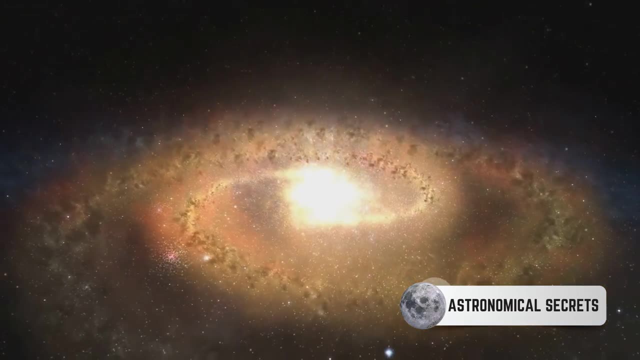 the galaxy's star-studded structure. In addition, these galaxies have a halo of dark matter surrounding them. This invisible substance doesn't emit light or energy, making it incredibly difficult to detect. However, its gravitational effects on the stars and galaxies are incredibly. 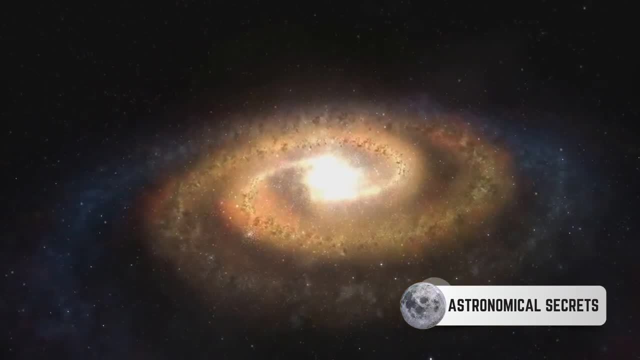 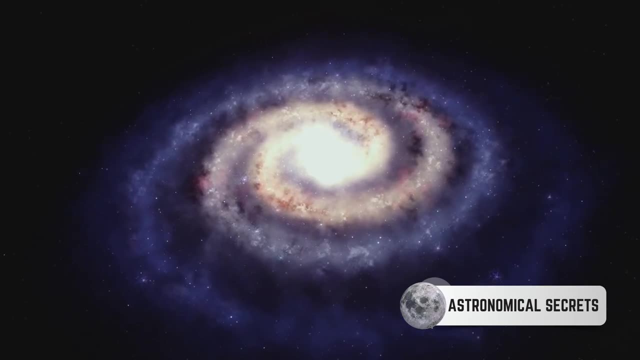 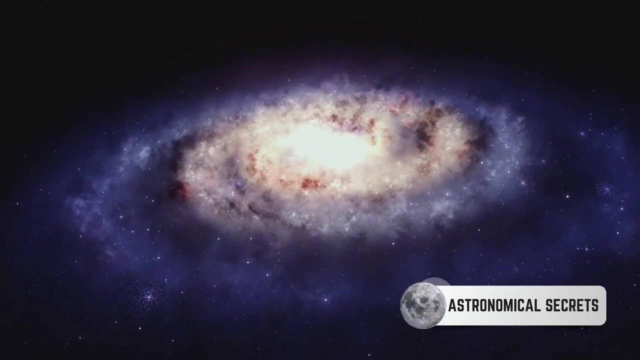 powerful and they can be easily detected. These galaxies may lack the flashy spiral arms of their counterparts, but their sheer size and star-packed structure make them a fascinating subject of study. They are the silent yet colossal players in the grand cosmic game, each holding secrets that can help us. 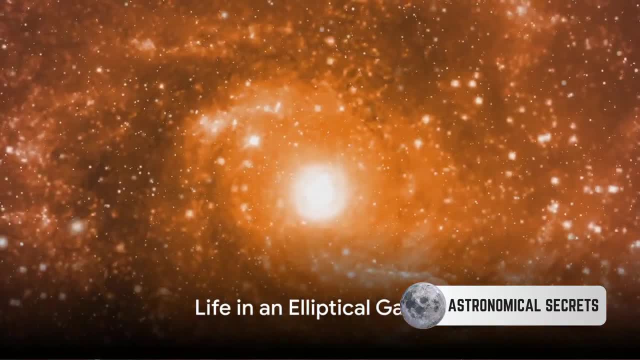 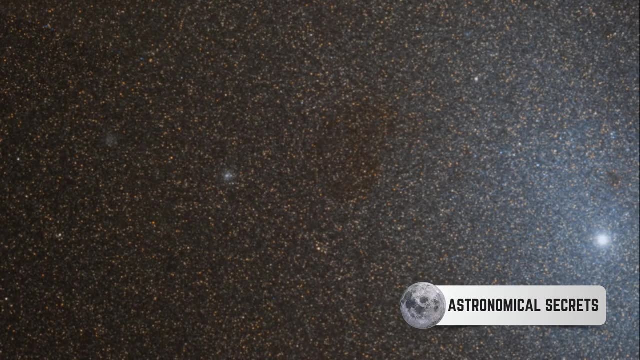 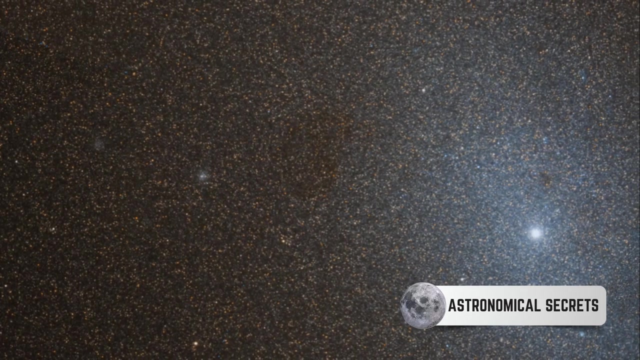 unravel the mysteries of the universe. Imagine living in an elliptical galaxy where the night sky is filled with a trillion stars. The concept might seem straight out of a science fiction novel, but let's dive into this thought experiment and explore it Now. an elliptical galaxy is a hotbed of ancient stars. These galaxies are shaped like elongated 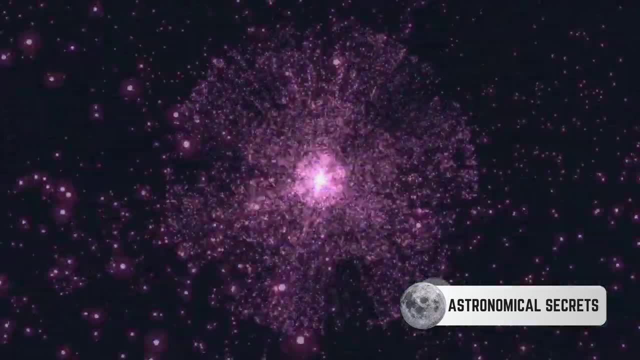 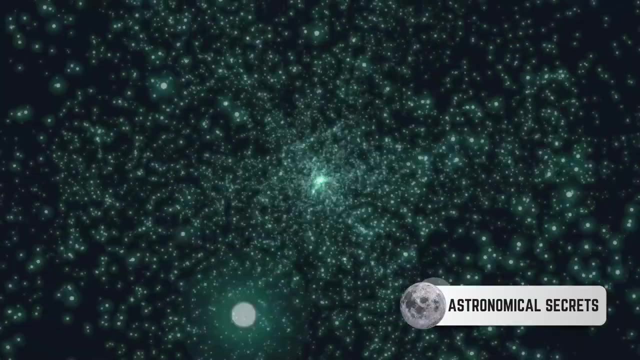 spheres, hence the name- elliptical. They are densely packed with stars, so if you were to gaze up at the night sky from a planet within one, it would be ablaze, with a spectacular stellar display. A trillion twinkling points of light- far more than our own night sky- would illuminate the 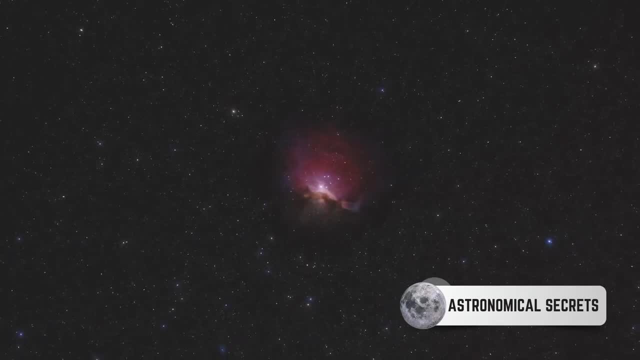 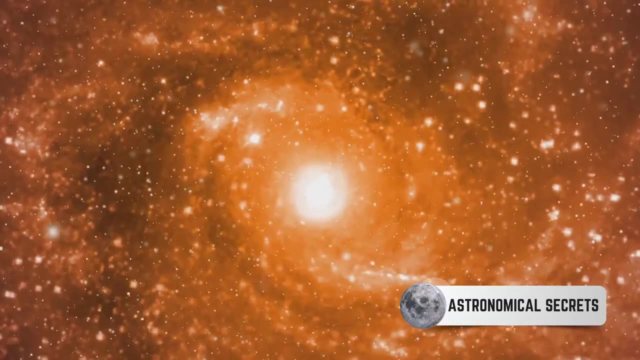 darkness. However, despite this breathtaking display, life in an elliptical galaxy would be quite different from that of an elliptical galaxy. So let's explore the implications of an elliptical galaxy from what we're familiar with in our Milky Way. You see, elliptical galaxies are largely devoid of the gas and dust necessary for new star formation. 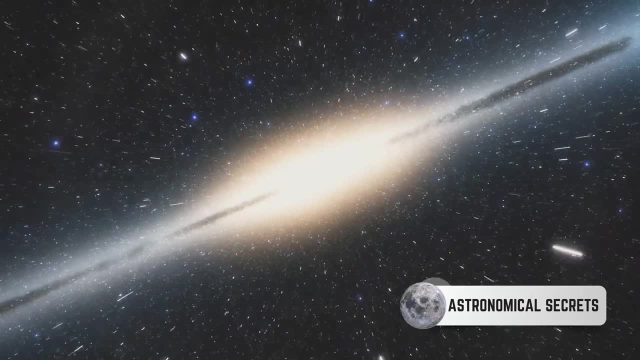 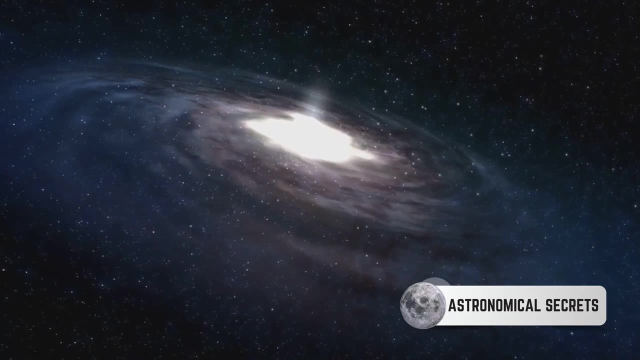 They are celestial retirement homes, if you will, where stars live out their twilight years. So what does this mean for potential life? Well, without new stars, there would be fewer opportunities for planets to form. Planets as we understand them are born from the dust and 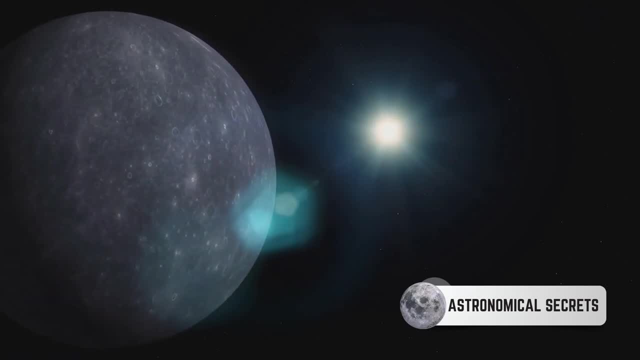 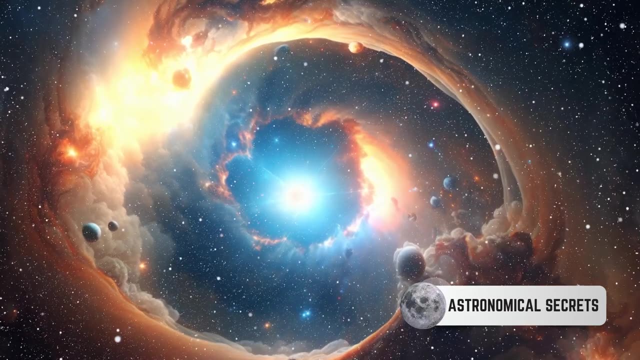 gas left over after a star is formed. No new stars, no new planets. Additionally, this lack of star formation would have other implications In our galaxy. the death of massive stars and supernova explosions is a crucial factor in spreading heavy elements necessary for life, as 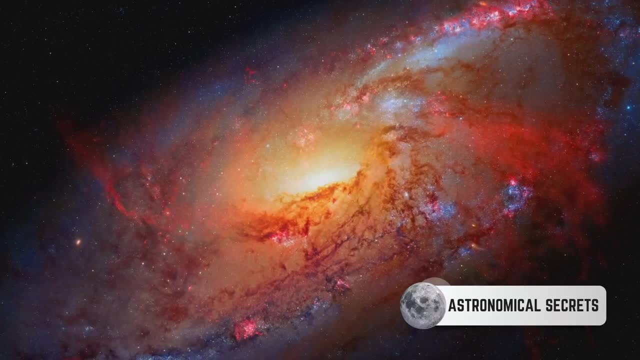 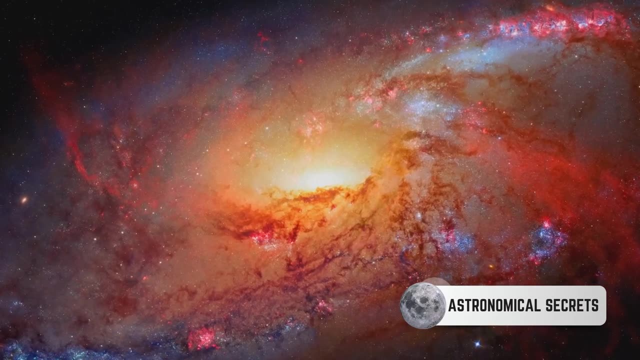 we know it, These elements, such as carbon, nitrogen and oxygen, are cooked up in the cores of massive stars and then scattered across the galaxy when the star explodes. In an elliptical galaxy with less star formation and hence fewer supernovae, these life-giving 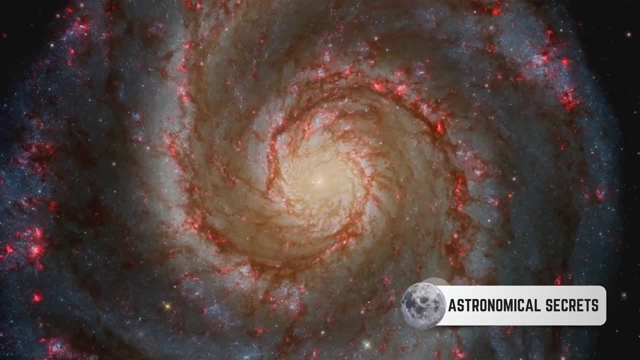 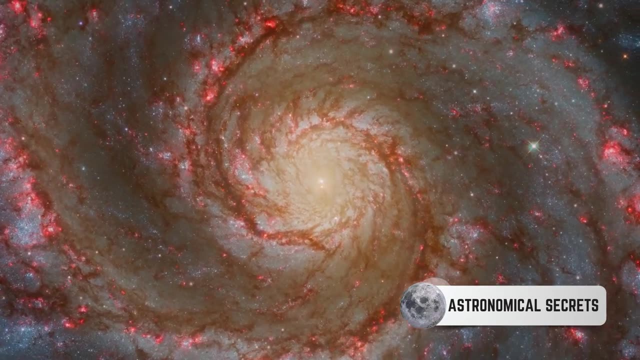 elements would be less abundant. All these factors combined suggest that while life in an elliptical galaxy is not impossible, it would be rare and potentially quite different from life as we know it. Life in an elliptical galaxy would be drastically different from life in our own Milky. 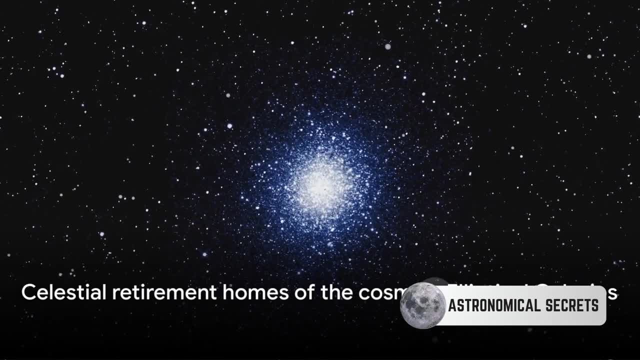 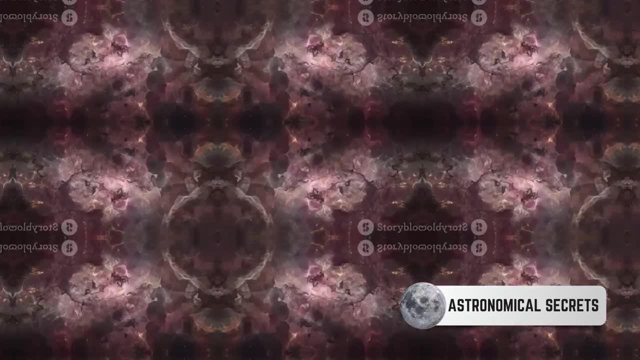 Way. So the next time you gaze up at our relatively calm and star-filled Milky Way, spare a thought for the celestial retirement homes of the cosmos: the elliptical galaxies. Elliptical galaxies are a cosmic mystery just waiting to be solved. 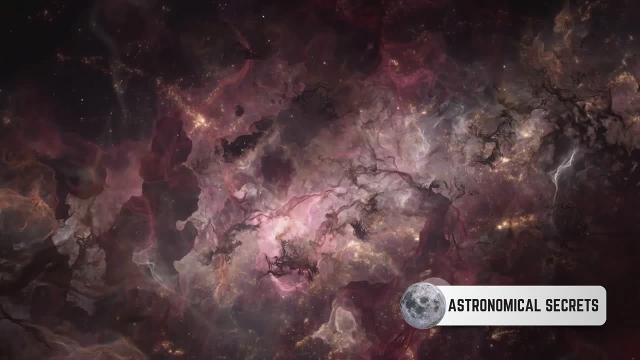 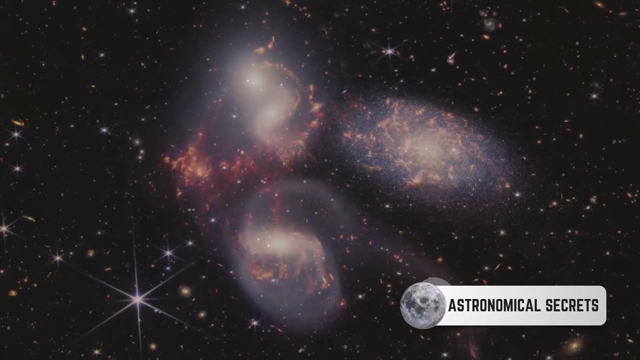 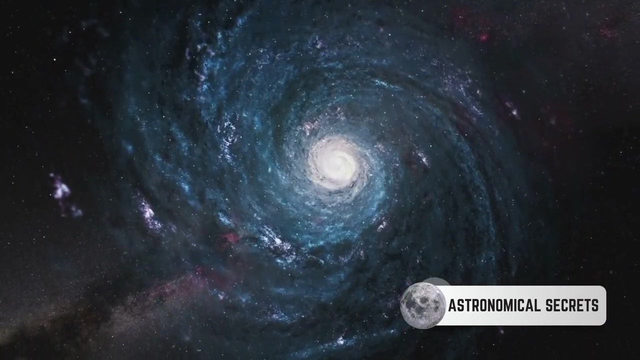 These celestial giants, teeming with old stars and sparse in cosmic dust, are a puzzle that scientists have been trying to piece together for decades. Unlike their spiral counterparts, elliptical galaxies seem to have stopped birthing new stars, But why? This is a question that has left astronomers scratching their heads. 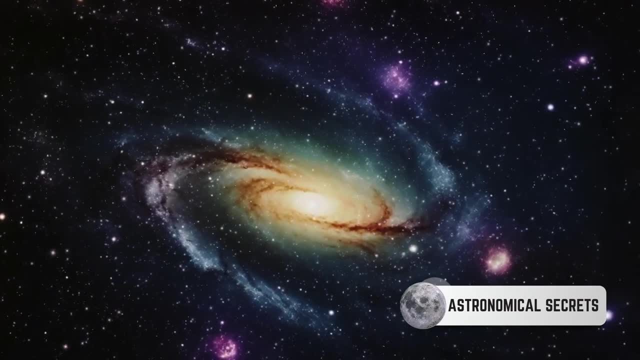 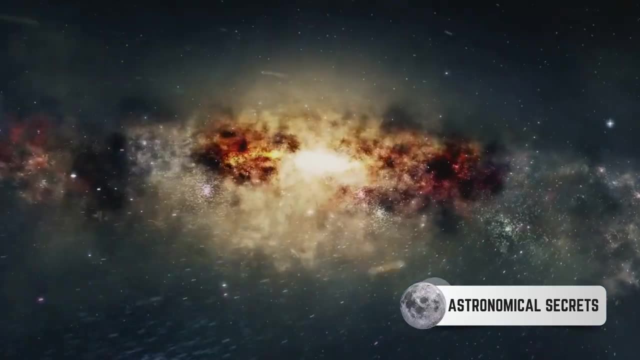 The lack of star formation in these galaxies is intriguing. Typically, galaxies are teeming with clouds of gas and dust, the essential ingredients for star creation. However, elliptical galaxies are noticeably lacking in these ingredients. It's as if they've suddenly lost their culinary 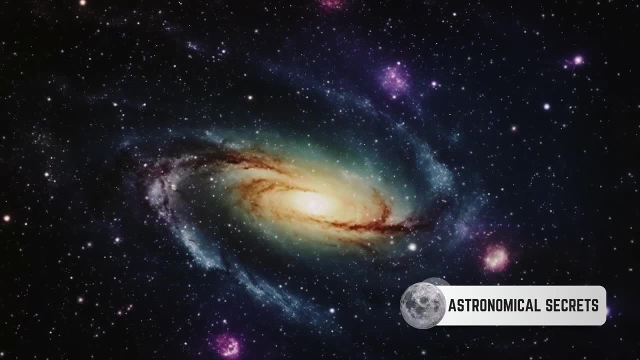 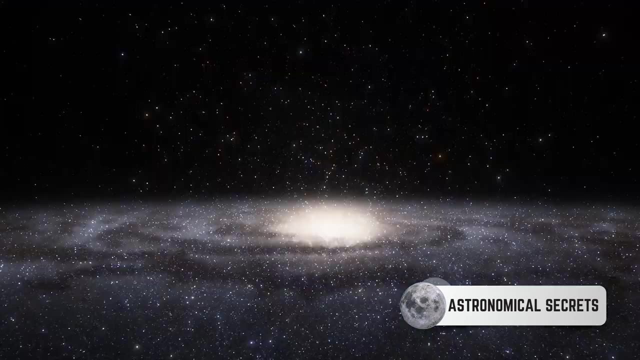 flair for making stars, But the question remains: where has all the gas and dust gone? Another mystery that baffles scientists is the sheer size of these elliptical galaxies. Some of them are colossal, dwarfing even the grandeur of the Milky Way. How did they grow? 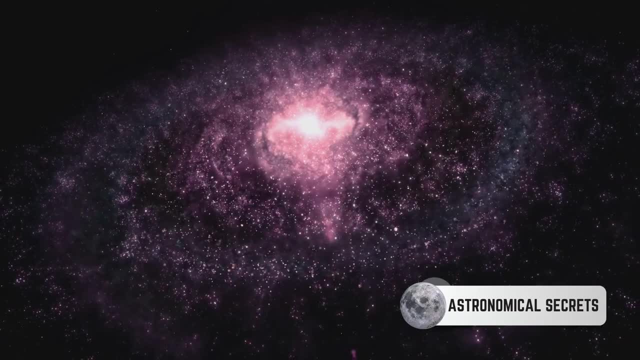 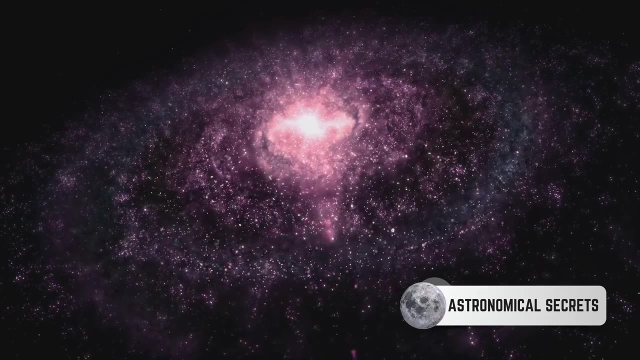 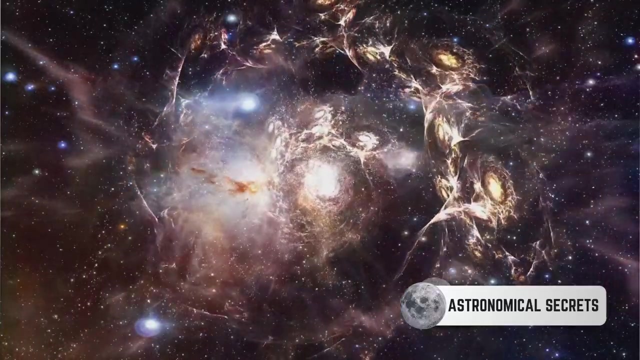 so large. One theory suggests that elliptical galaxies are the result of cosmic collisions. When smaller galaxies collide and merge, they could potentially form these massive star-filled spheres, But this is just a theory, And the exact process. The answer to this question remains elusive Despite these unanswered questions. 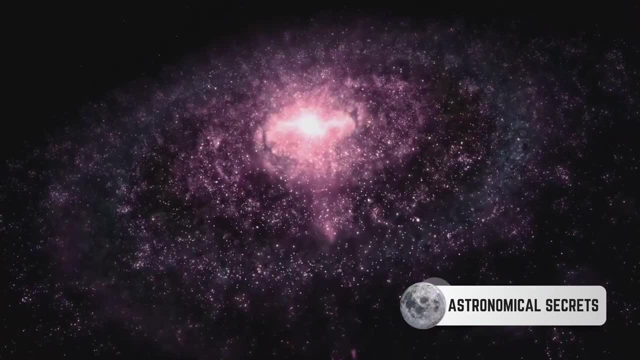 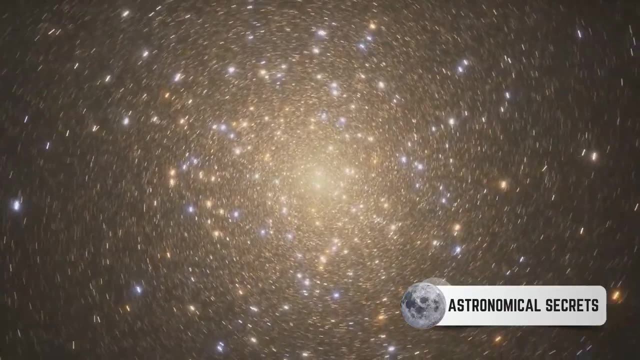 we know that elliptical galaxies are not just cosmic anomalies. They are a testament to the ever-changing dynamic nature of the universe. They are proof that the cosmos is not a static place but a vibrant, evolving entity. The mysteries surrounding elliptical galaxies: 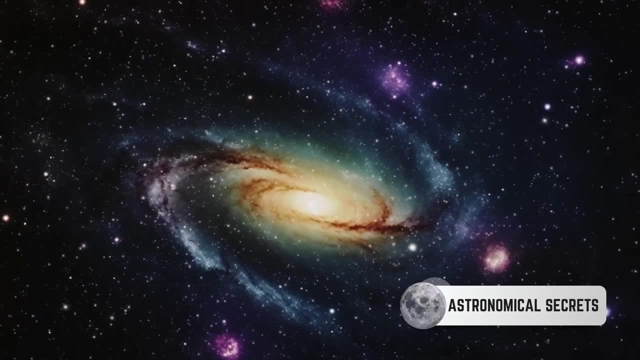 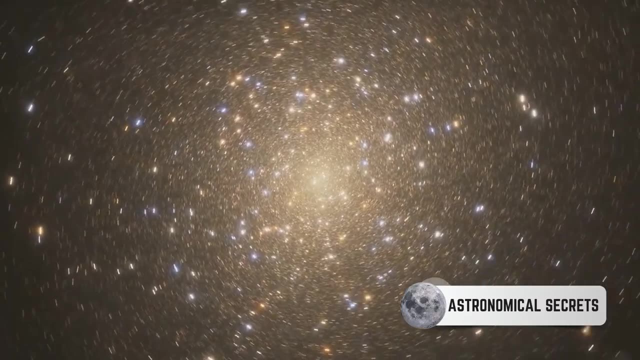 are far from being fully understood. With every passing year, new discoveries are made and we inch closer to deciphering the secrets of these grand cosmic entities. And though many questions remain unanswered, the pursuit of knowledge continues After all, the beauty of the cosmos. 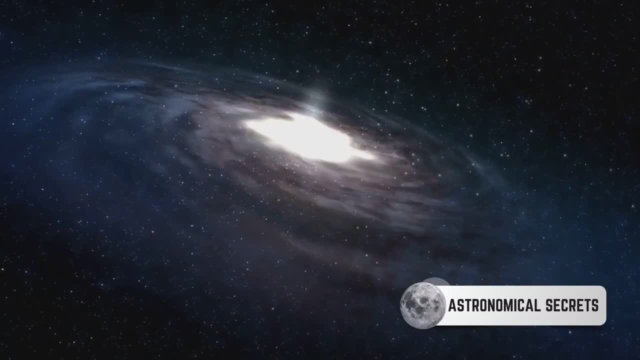 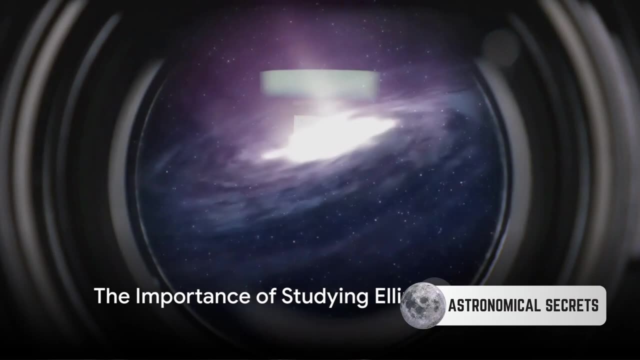 is not just in the answers we find, but also in the questions we ask As we continue to study these cosmic giants. who knows what secrets we'll uncover? Studying elliptical galaxies isn't just about satisfying our cosmic curiosity. it's about understanding the universe itself. 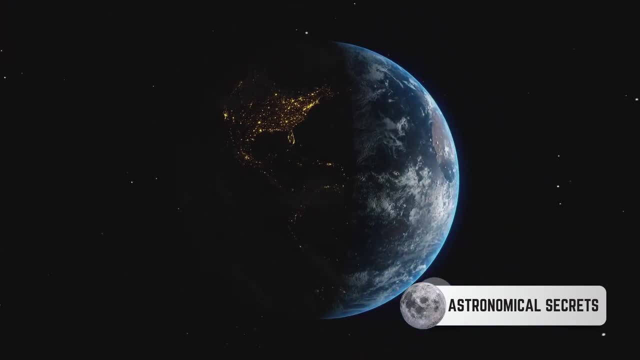 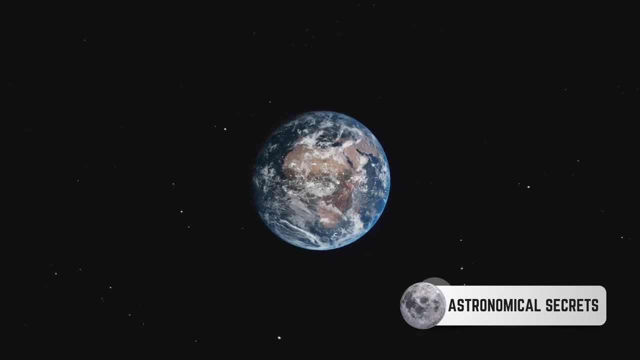 Imagine that the universe is a grand cosmic puzzle. Each galaxy, planet and star is a unique piece that helps us see the bigger picture. Among these pieces, elliptical galaxies hold a special place. They are the sleeping giants of the cosmos. 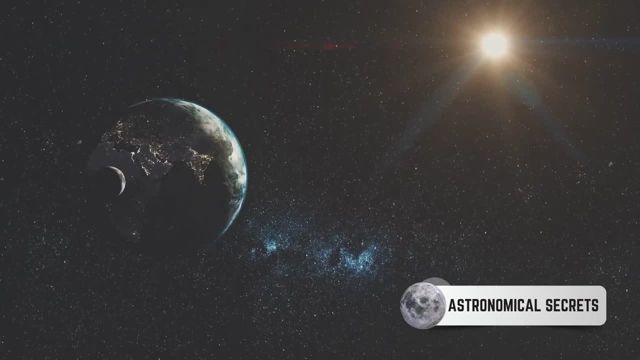 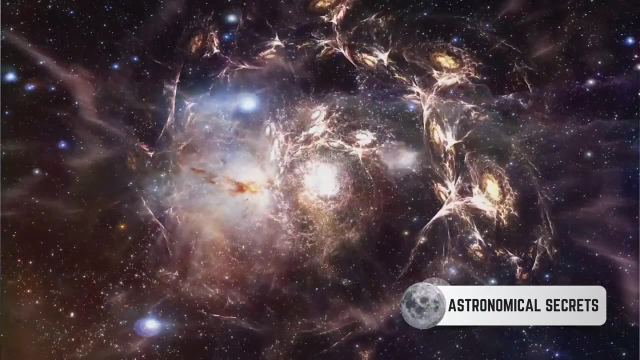 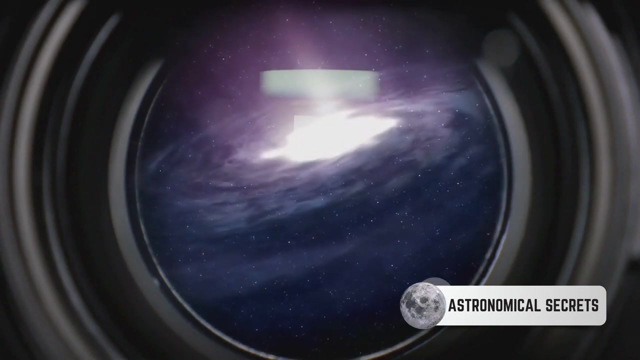 holding secrets that can drastically change our understanding of the universe. Elliptical galaxies serve as cosmic laboratories for astronomers. By studying these galaxies, scientists can gain deep insights into galaxy formation and evolution. These galaxies are often the oldest in the universe, having witnessed billions of years. 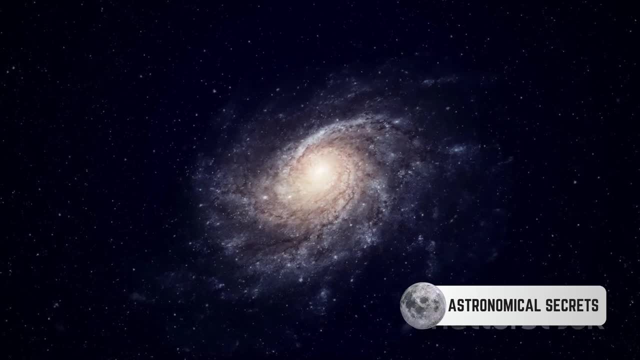 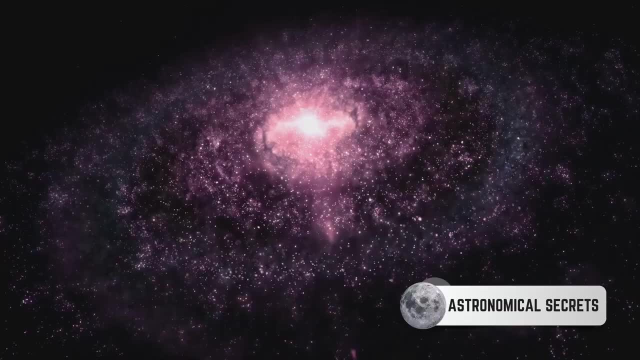 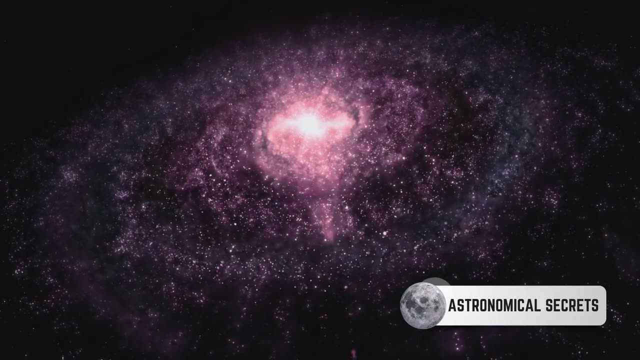 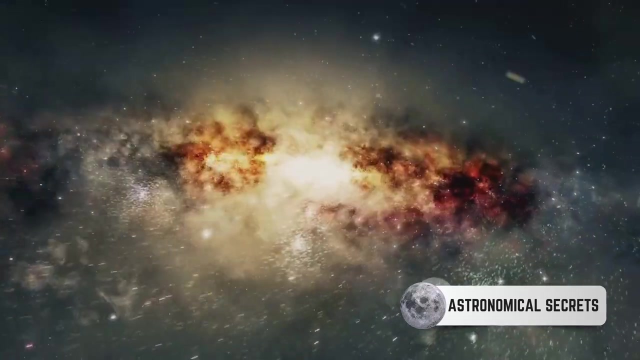 changing and evolving over unimaginable spans of time. Moreover, elliptical galaxies can provide clues about one of the most elusive substances in the universe—dark matter. The gravity of these galaxies, which is far greater than can be explained by the visible matter, they contain hints at the presence of this mysterious substance. Studying the 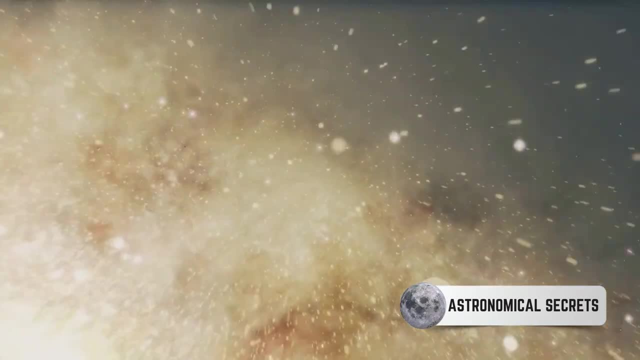 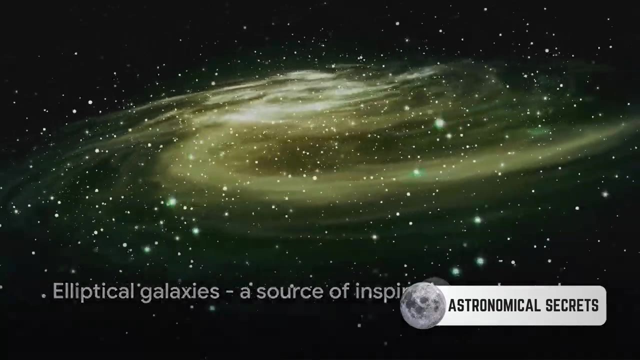 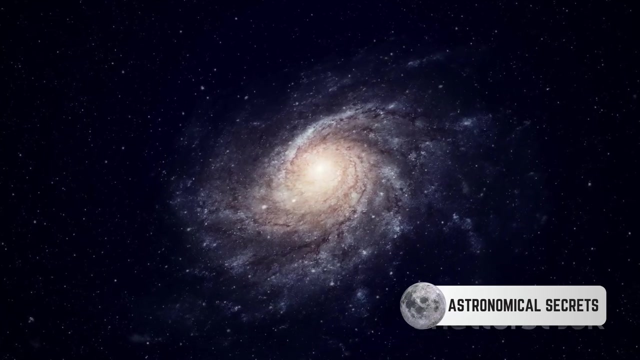 distribution and behavior of dark matter within these galaxies can help us understand its nature and its role in the universe. But the importance of studying elliptical galaxies goes beyond the purely scientific. These galaxies challenge our imaginations, inspire our creativity and expand our sense of wonder. They remind us of the vastness of 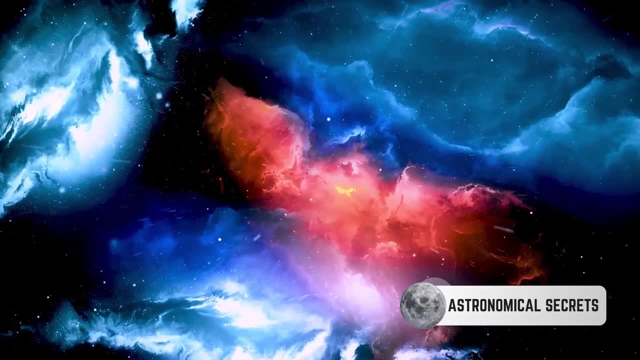 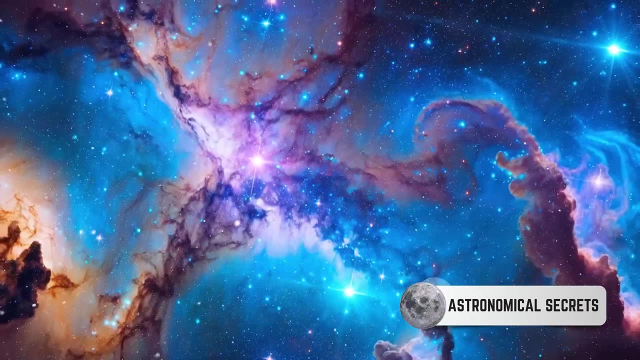 the universe and our small yet significant place within it- And let's not forget, every discovery we make about elliptical galaxies- also has the potential to impact our technology, our culture and our future. Who knows what new technologies or ideas might be sparked by our growing 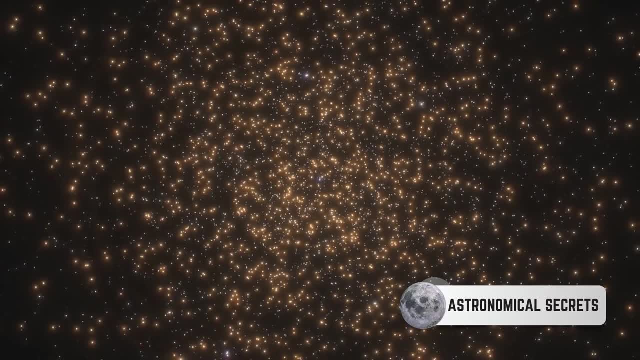 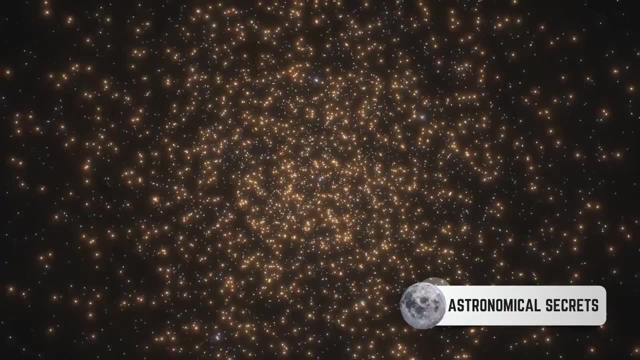 understanding of these cosmic giants. In the end, studying elliptical galaxies isn't just about learning more about the stars. It's about seeking answers to some of the biggest questions we have about our existence and our universe. It's about continuing our journey of discovery and 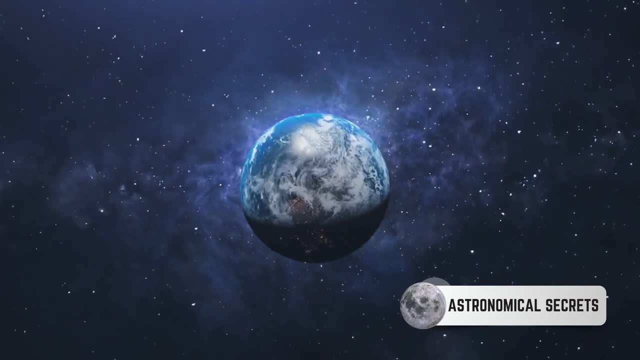 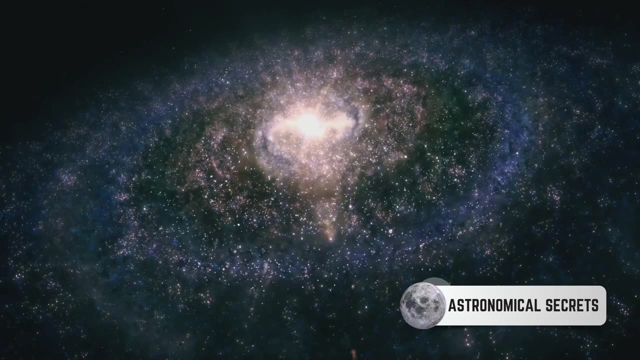 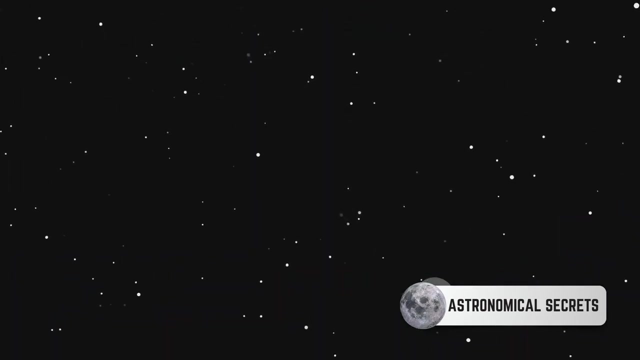 exploration, pushing the boundaries of our knowledge and our imagination. Every bit of information we glean from these sleeping giants brings us one step closer to understanding our place in the cosmos. So there you have it, The sleeping giants of the cosmos, elliptical galaxies. We've journeyed from their enigmatic structure shining a.